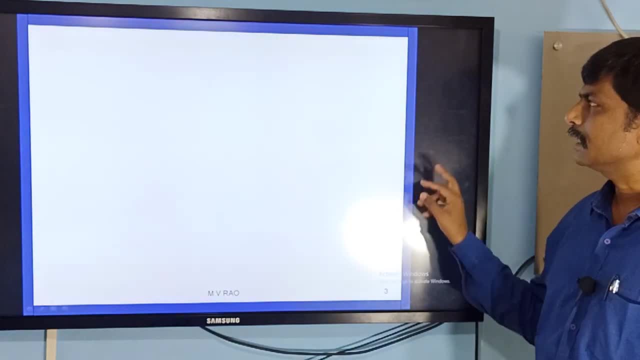 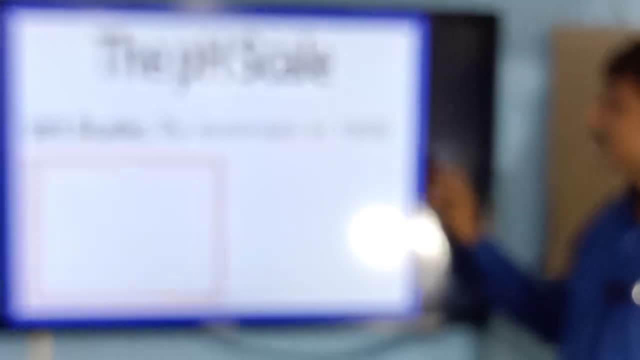 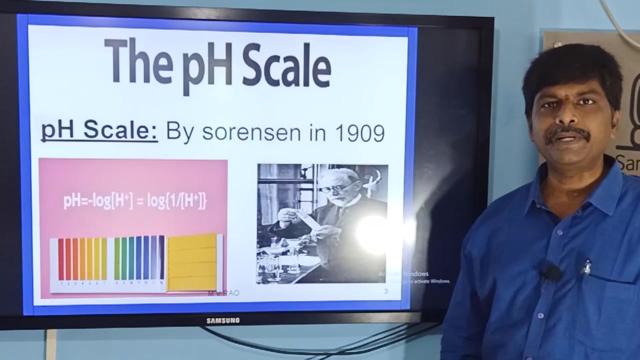 activities. Now in this class I am going to explain about pH scale. pH scale is discovered by Sorensen in 1909. Sorensen discovered pH scale. What is pH? What is meant by pH? 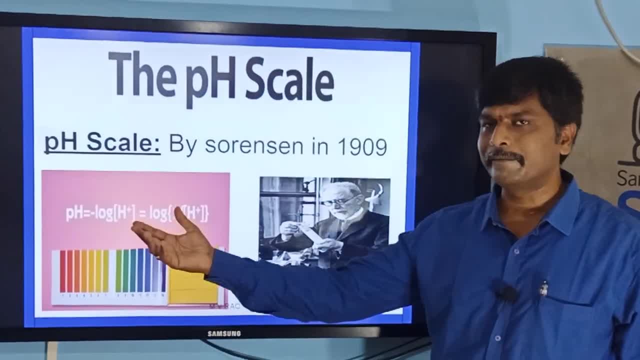 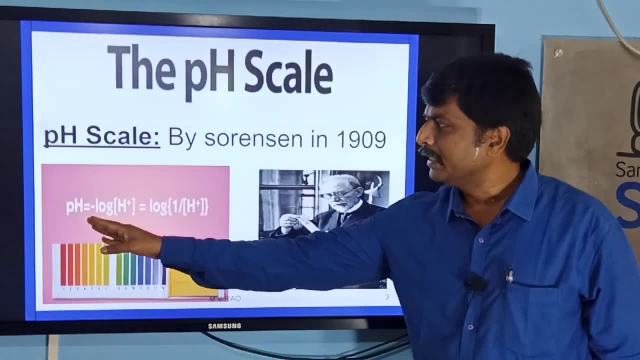 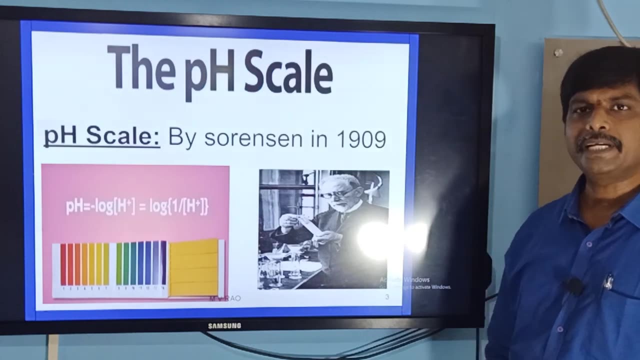 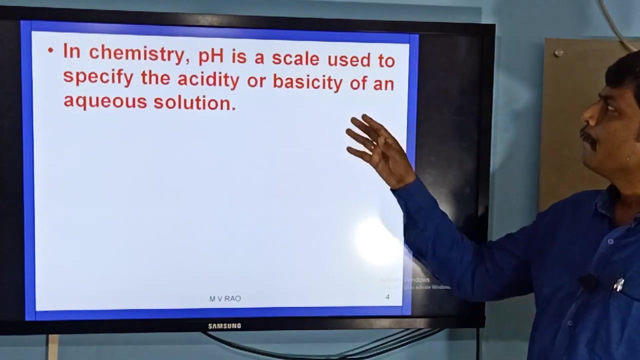 For it is difficult. So it will come in class 11. pH is negative logarithm of hydrogen ion concentration. The negative logarithm of hydrogen ion concentration is called pH. What is pH? The negative logarithm of hydrogen ion concentration is called pH. In chemistry pH is a scale used to 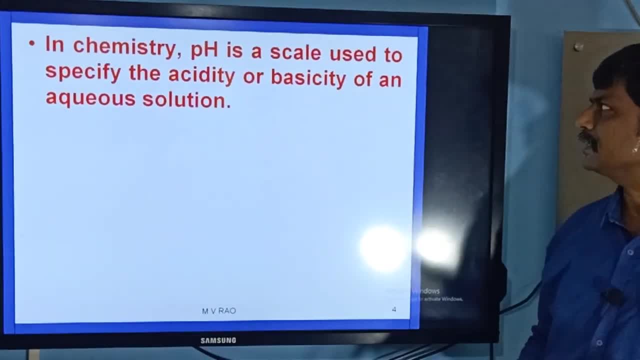 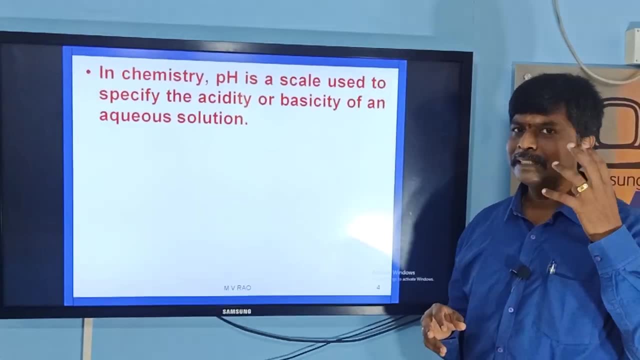 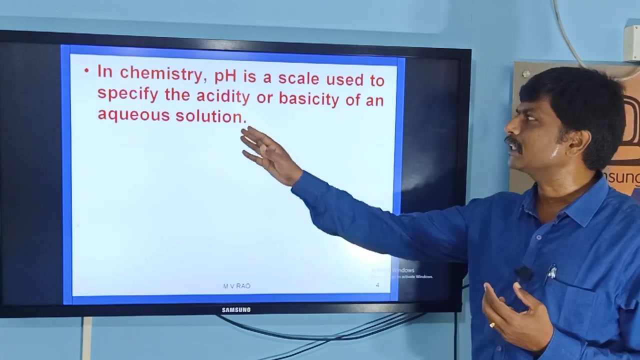 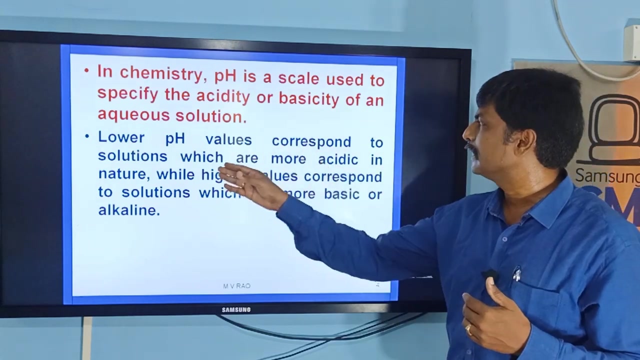 specify the acidity or pH. The basicity of an aqueous solution. If you want to know the pH you want to know the nature of the solution. Whether the given solution is acidic or basic. If you want to know this pH concept is needed. So lower pH values. pH values if you are lower less than that solutions are more acidic. 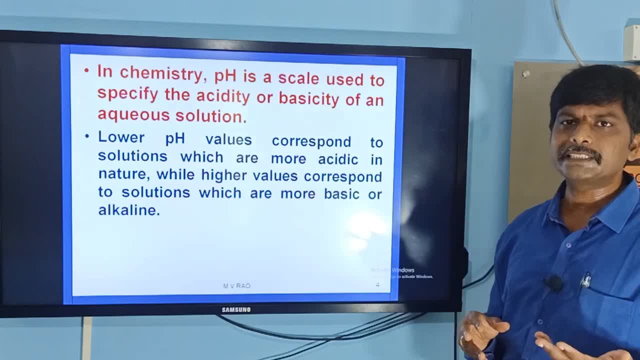 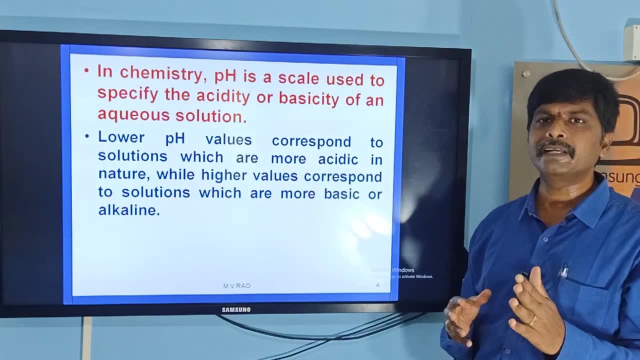 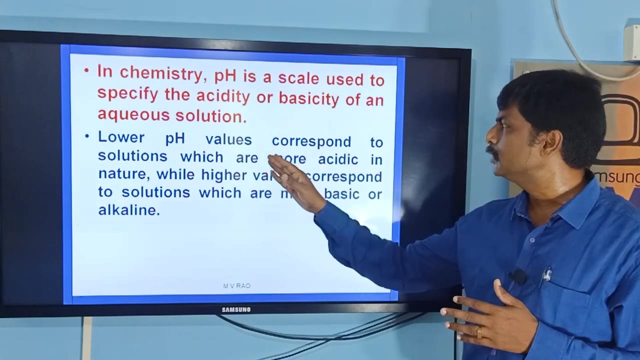 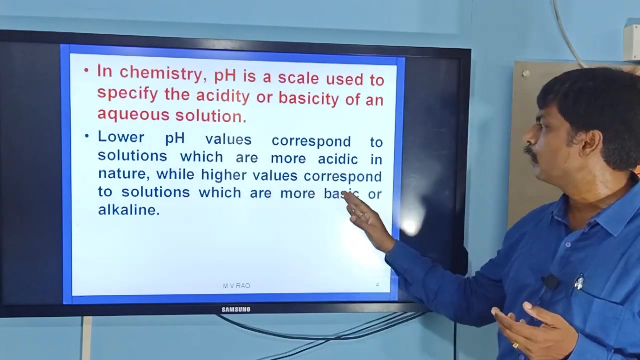 Actually pH is less than seven. That solutions are acidic. So pH is greater than seven. that solutions are basic ph is exactly equal to 7 that the nature of the solution is neutral lower ph values correspond to solutions which are more acidic in nature while higher values correspond to solutions which are more basic or alkaline at room temperature pure water is 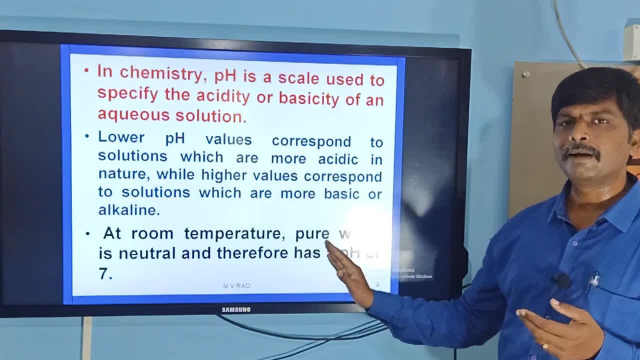 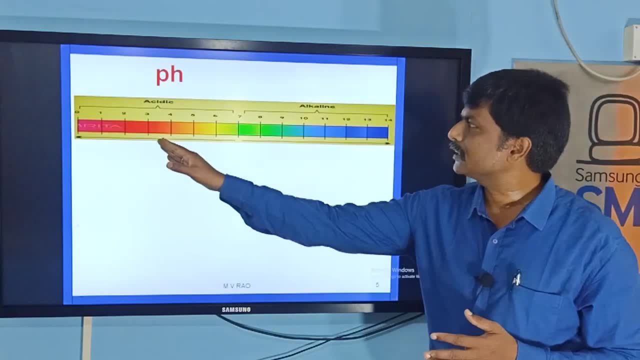 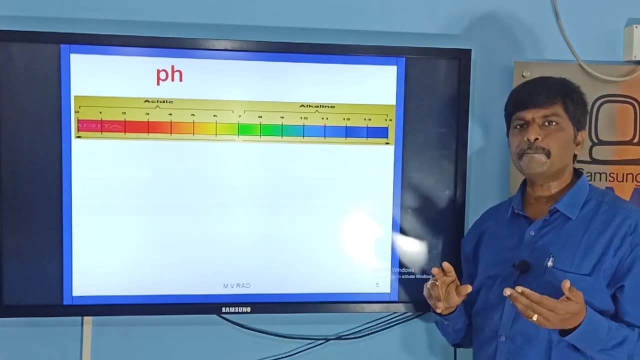 neutral and therefore as ph of 7 for neutral solutions what is the ph is equal to 7 now ph it is the ph scale what is the range of ph scale it starts from 0 to 14 what is the range of ph scale 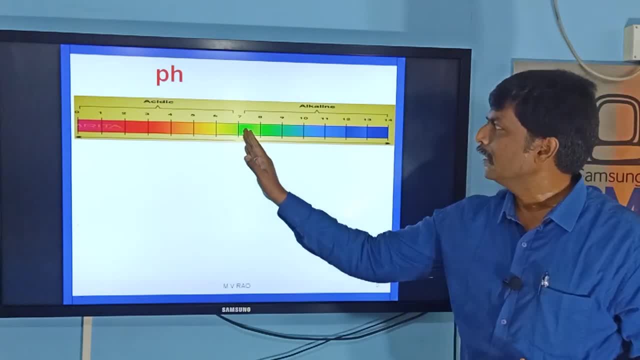 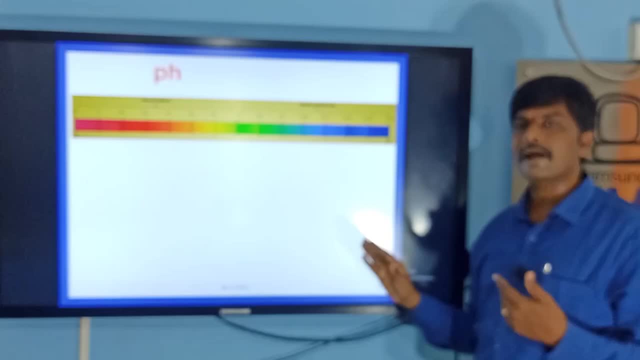 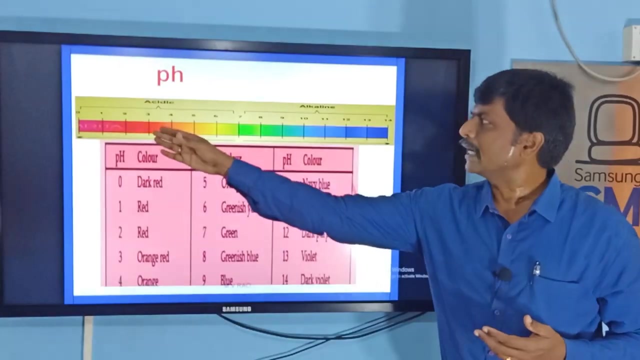 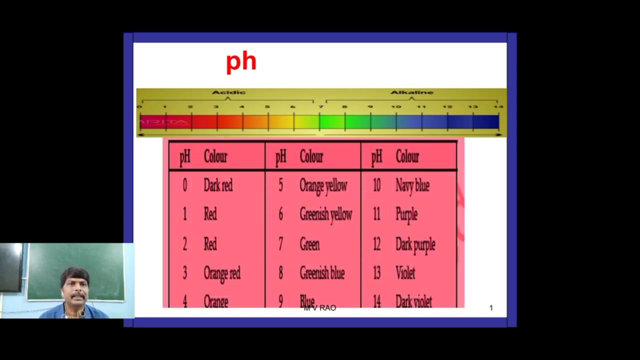 0 to 14 from 0 to 7 the nature of the solution is acidic 7 to 14 the nature of the solution is basic if it is 7 the nature of the solution is neutral so in this actually it is the universal indicator colors so it is universal indicator ph paper universal indicator exhibits different colors 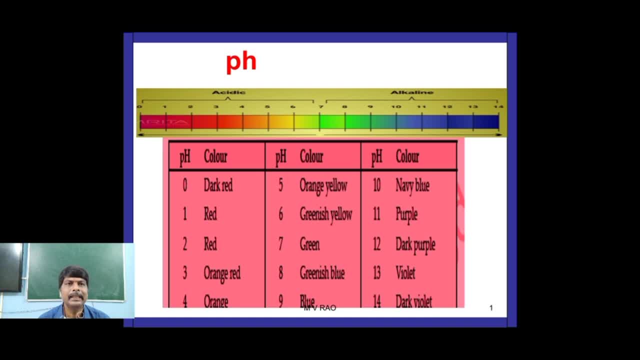 at different ph values for example you see here at ph0 its color is dark red at ph1 red at ph2 red at ph3 orange red at ph4 orange at ph5 orange yellow at ph6 greenish yellow at ph7 green at ph8 greenish blue at ph9 blue at ph10 navy blue at ph11 it exhibits purple color at ph12 it exhibits dark purple color ph 13 violet ph 14 dark violet that means 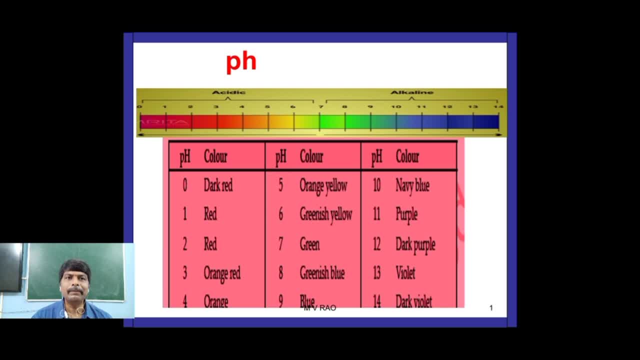 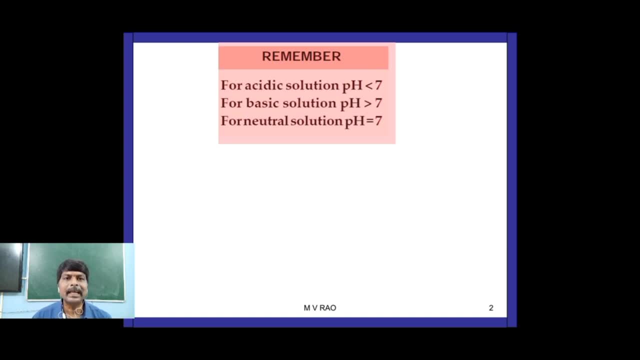 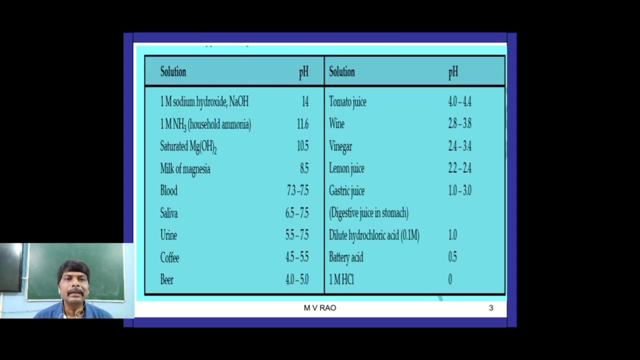 means universal indicator exhibits different colors at different pH values. One more point from pH scale you can say if pH is less than 7 that the nature of the solution is acid. For basic solutions pH is greater than 7. For neutral solutions pH is equal to 7. You can see here in this pH scale if it is 7 neutral it is coming down from 7 to towards 0 7 to 0 towards 0 pH decreases that means increasing of acidic character increasing of acidic character as pH value decreases acidic nature increases. In the other hand 7 to 14 while moving from 7 to 14 pH value increases. pH value increases means basic character increases basic character increases. Here some examples given from this pH values you can see nature of that solutions actually it is related to one activity from our textbook. You take 1 molar sodium hydroxide. 1 molar sodium hydroxide means it is a base base. Alkali sodium hydroxide means it is a base. Alkali sodium sodium hydroxide is an example for strong base. What is its pH? 14. Base means its pH is anyway greater than 7. It is strong base so that's why its pH is 14. One more example 1 molar NH3. 1 molar NH3 household ammonia solution. Ammonia solution. So its pH is 11.6 so that means it is also basic. Next one is milk of magnesium. That means two types are there here saturated MgOH2. Saturated MgOH2 means it is strong. Magnesium hydroxide its base is 10.5. Milk of magnesium base it is also base mild base. Its base pH value is 8.5. Blood what is the pH of blood. Its range is 7.3 to 7.5. Saliva pH is 6.5 to 7.5. Urine pH is 5.5 to 7.5. Coffee is acidic in nature. So you take more coffee then you will get acidity problem. So what is the pH? 4.5 to 5.5. Beer that alcohol it is also pH is 4 to 5. Next tomato juice 4 to 4.4. Wine 2.8 to 3.8. Vinegar 2.4 to 3.4. Lemon juice 2.2 to 2.4. Grass fruit juice 1 to 3. So dilute hydrochloric acid almost 1 because it is a strong acid. And next one is butyric acid, battery acid that means sulfuric acid. It is strong acid. Its pH is 0.5. 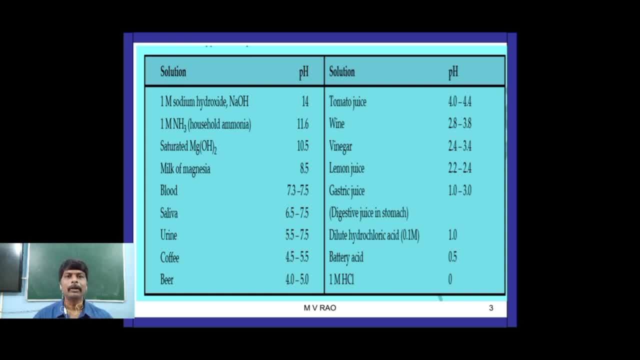 1 molar is Cl. Its pH is 0. So you have to remember pH values of these substances like example coffee and vinegar, lemon juice, gastric juice. These questions will come per multiple 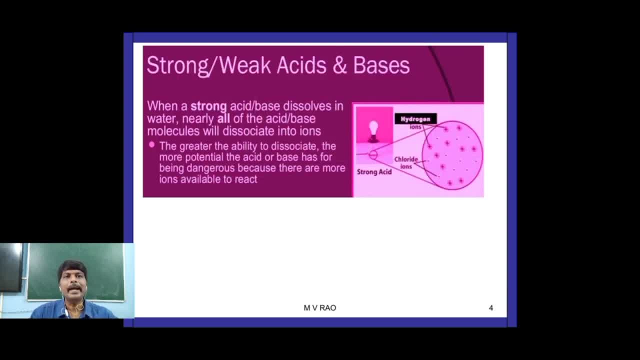 choice questions in our exams. Now what is meant by strong acid? What is meant by weak acid? Strong base, weak base already discussed in first class. Again I will explain today. So what is meant by strong acid? 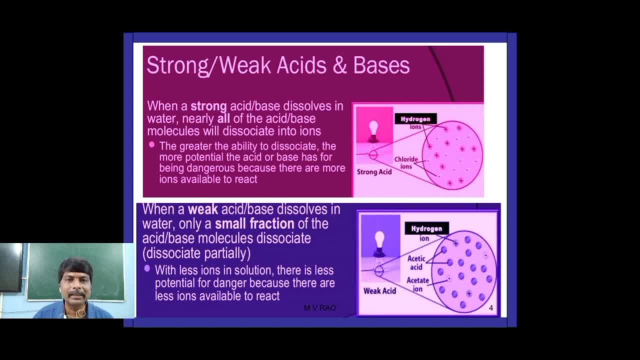 Strong acid which gives more number of H plus ions in water. Acid which gives more number of H plus ions in water is called strong acid. You can define in another way that is completely ionized. Acid 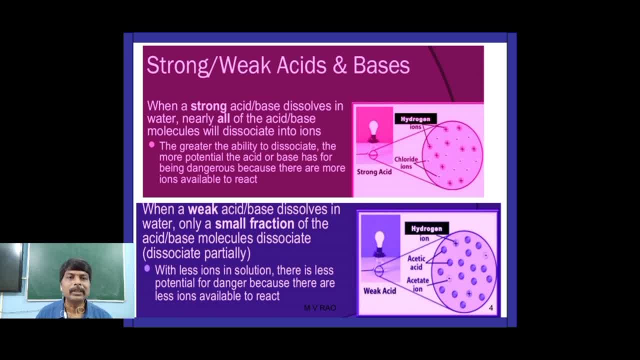 which undergo complete ionization, which undergo complete ionization is strong acid. So that is why it is a good conductor of electricity. Strong acids and strong bases are good conductors of 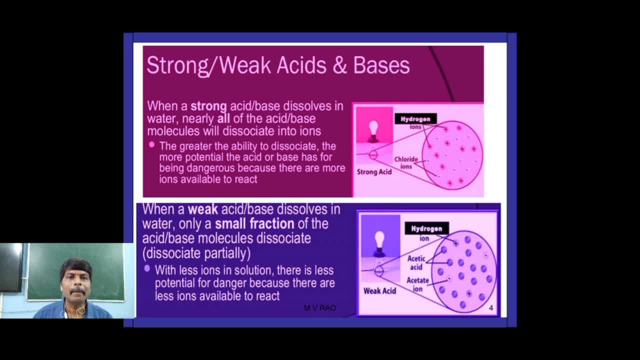 electricity because they undergo complete ionization. What is meant by weak acid? Weak acid means 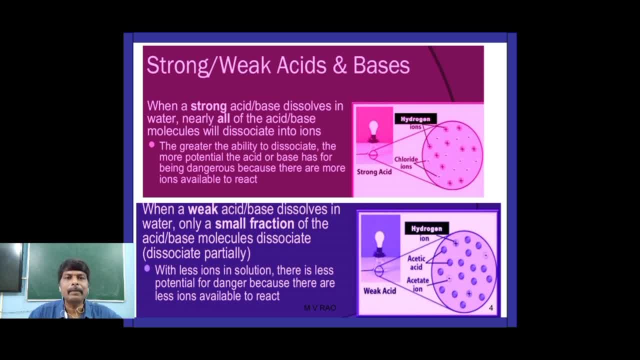 the substance which gives less number of H plus ions in water is called weak acid. The substance which gives less number of OH minus ions in water is called weak base. So another way is partially ionized. The 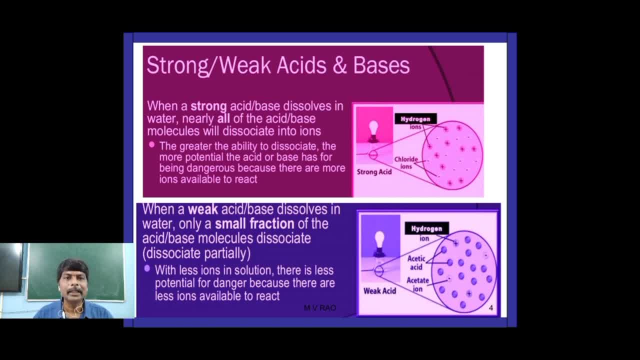 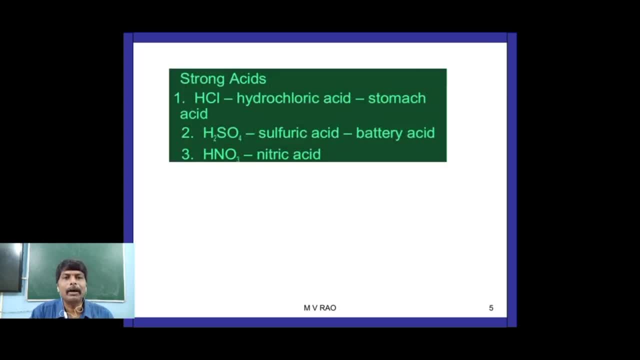 partial ionization complete ionization means strong acid partial ionization means weak acid here i will give some examples strong acids examples it is important to you have to memorize 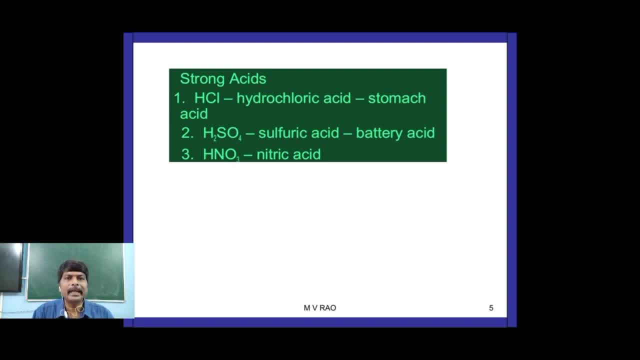 keep memory so hcl hydrochloric acid generally it is present in our stomach stomach acid it is 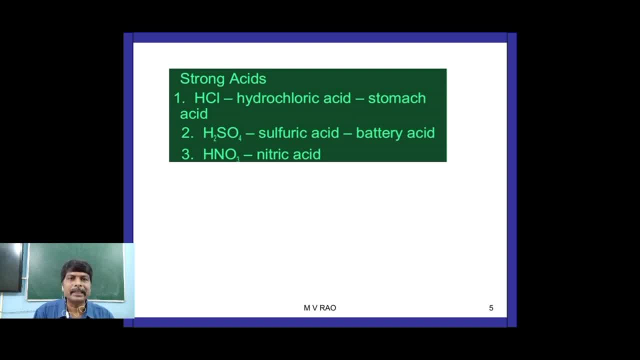 strong acid sulfuric acid battery acid it is king of chemicals formula is H2SO4 nitric acid it is also strong acid acetic acid vinegar its formula is CH3COOH citric acid you can find 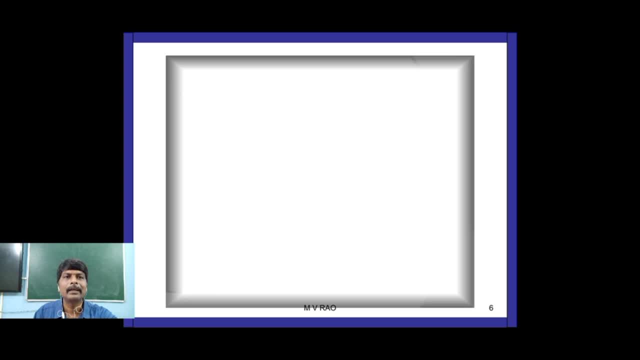 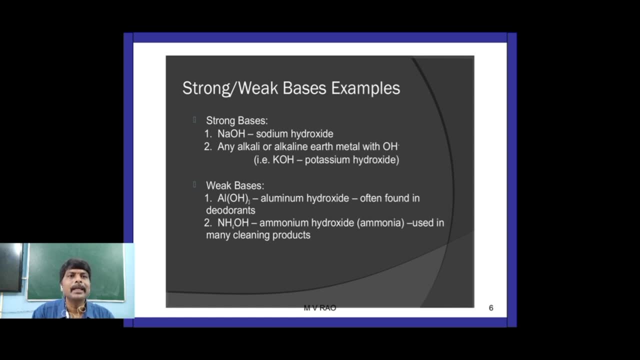 in citrus fruits it is also weak acid now you see strong base strong base sodium hydroxide sodium hydroxide is strong base any alkali or alkaline earth metal with OH alkali metal means group 1 element 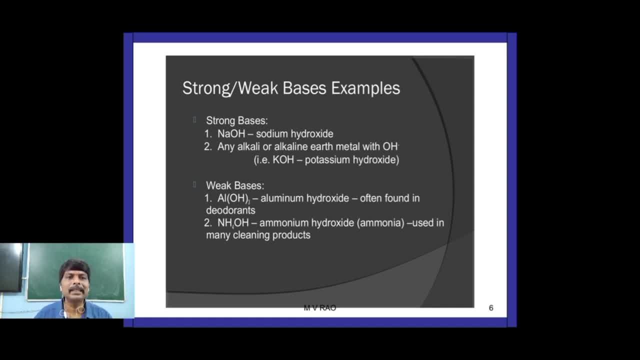 in the periodic table what are the elements in group 1 what are the elements in group 1 lithium sodium potassium rubidium cesium transium these are the elements present in group 1 so corresponding hydroxides acts as strong bases so that's why group 1 elements are called alkali 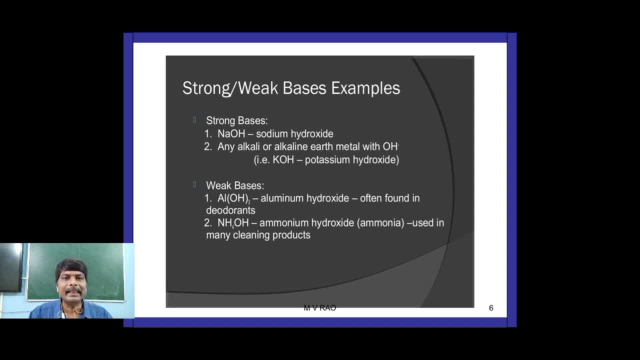 metals similarly alkaline earth metals alkaline earth metals are called alkaline earth metals metals means group 2 elements in the periodic table what are the elements beryllium magnesium calcium strontium barium and radium so these elements belongs to group 2 radium is the 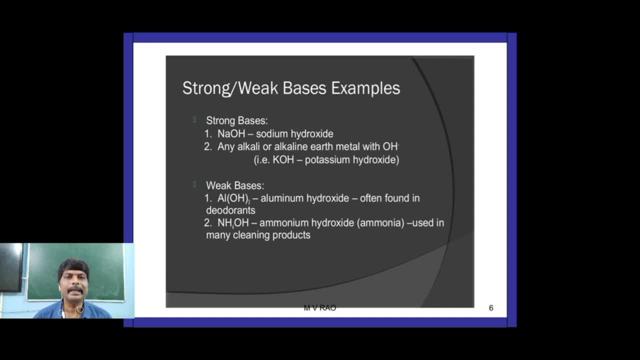 radioactive element other than radium the remaining elements are called alkaline earth metals strong bases means it may be related to either group 1 or group 2 general elements of aerodinamics and so forth there are a few other elements in the periodic table benzylam is a strong base material 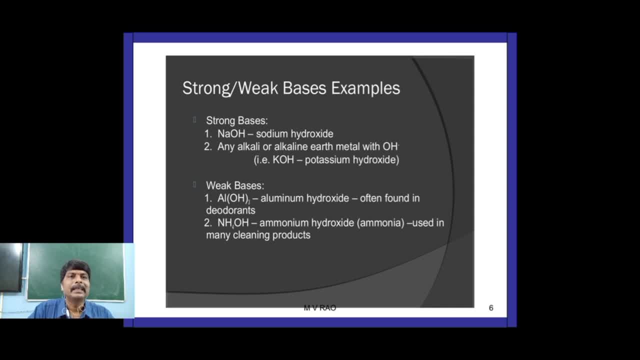 generally. What is meant by weak base? You already know, already I told you what is weak base? A substance which gives less number of OH minus ions in water. A substance which 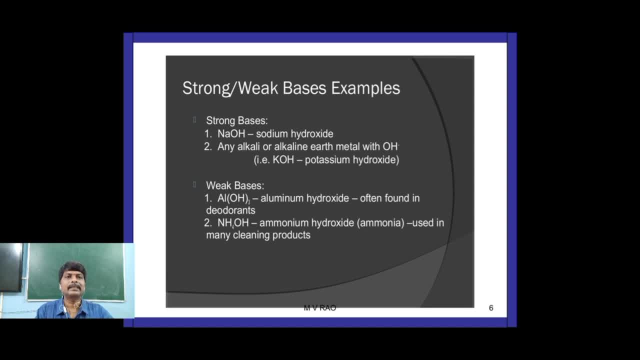 gives less number of OH minus ions in water is called weak base. Another form of definition is a base which undergo partial ionization is called weak base. What are the examples 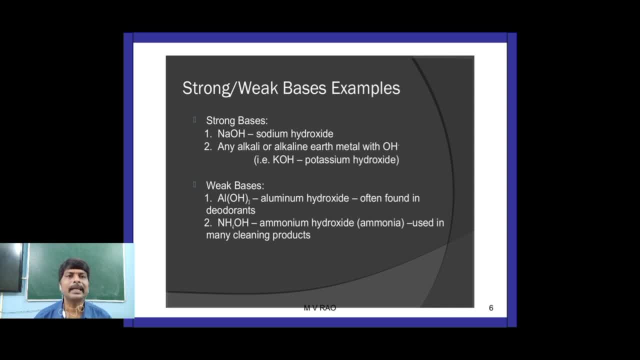 for weak bases? Aluminium hydroxide, AlOH3, aluminum hydroxide. Next, ammonium hydroxide, 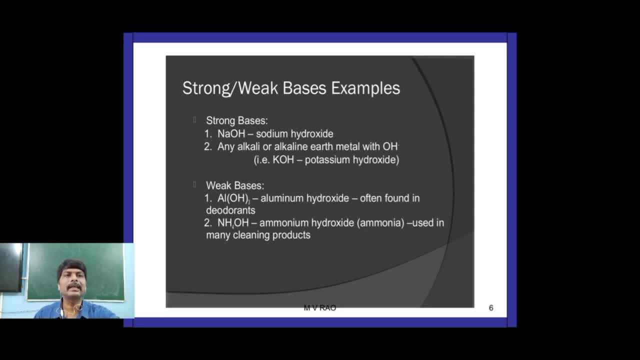 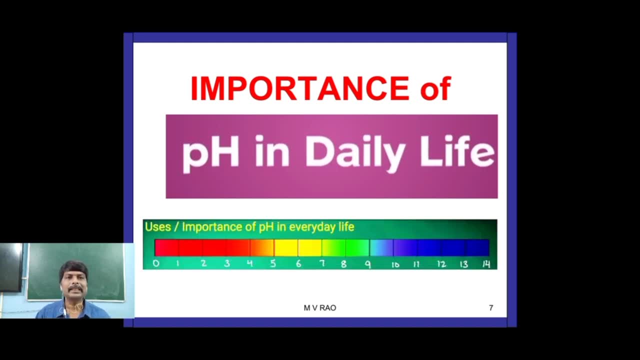 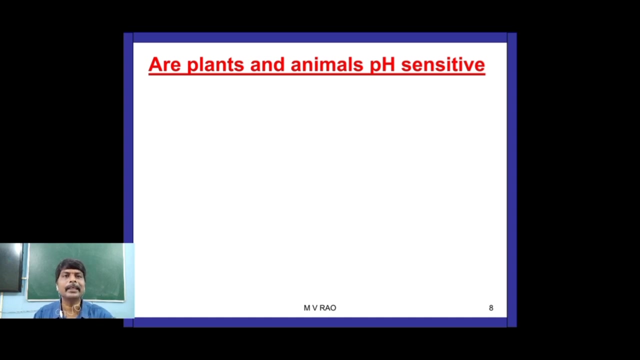 NH4OH. So, these are weak bases. Next one is importance of pH in daily life. So, it is important to know the importance of pH in daily life. So, it is important to know the importance of pH in daily life. So, it is important to know the importance of pH is for examination point of view. It is important topic. Uses, uses are importance of pH in everyday life. pH is playing an important role in our daily life and in nature also. 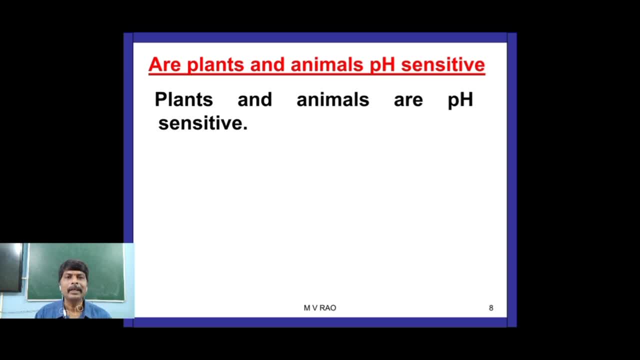 Are plants and animals pH sensitive? Is there any link between pH per plants, pH and animals? Yes, plants and animals are pH sensitive. 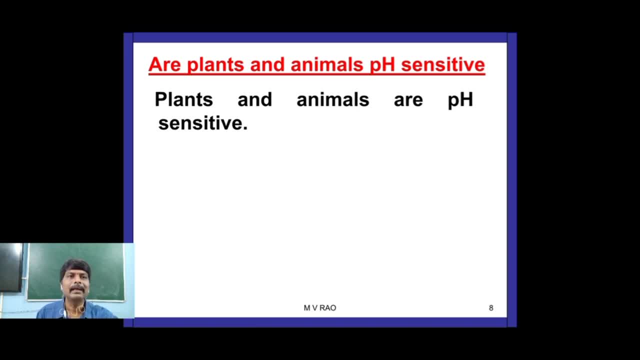 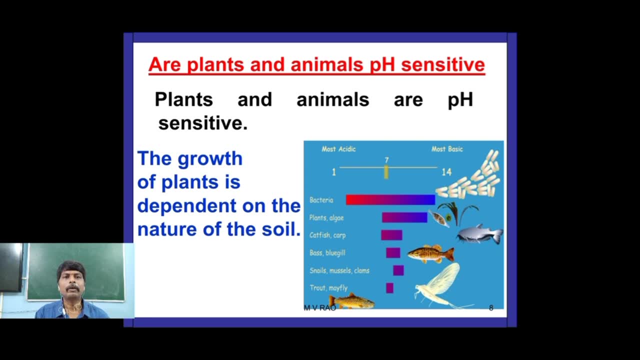 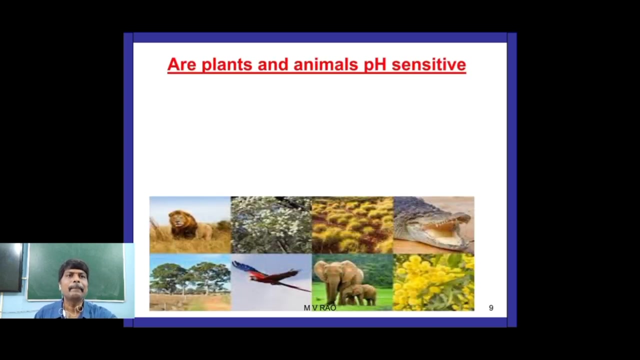 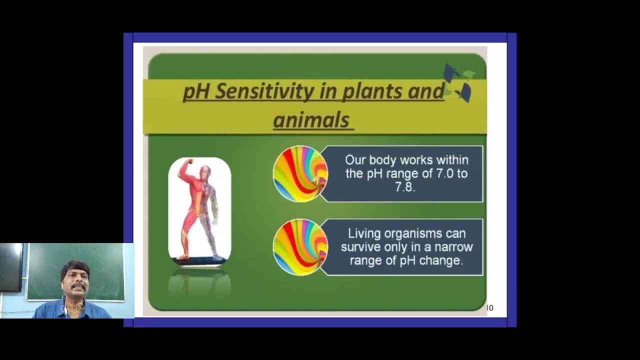 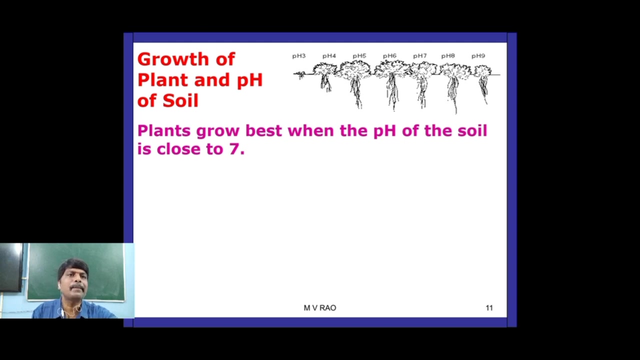 plants and animals are ph sensitive why you see plants and animals some examples the growth of plants the growth of plants is dependent on the nature of the soil so for the healthy growth of plant so good soil is required that means soil with certain ph value is essential so you say you take here plants and animals ph things so if the ph of the soil is greater than seven and it is called alkaline if it is greater than seven means base alkaline then the plants cannot grow in the soil if ph of the soil is greater than seven then that soil becomes alkaline like basic nature then the plants cannot grow in that type of soil when it comes to animals about soil power next when it comes to animals the ph level in their stomach needs to be maintained next for example you see our body works with ph range 7 to 7.8 next living organisms can survive only in a narrow range of ph now you see growth of plants and animals plants grow best when the ph of the soil is greater than seven and it is called alkaline so if the ph of the soil is close to seven if it is greater than seven it basic so if the soil is too acidic or too basic or alkaline then the plants cannot grow at all so soil naturally should be 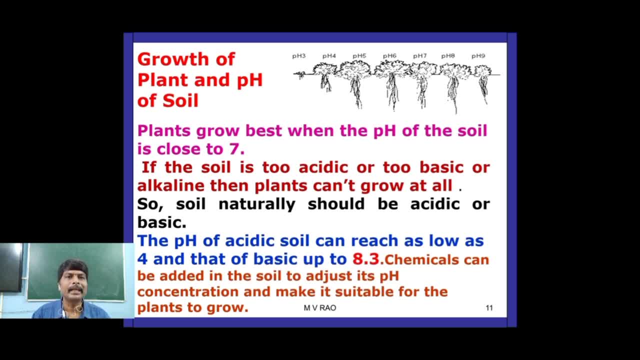 acidic or basic it is around seven only the ph of acidic soil if it is acidic then can reach as low as four then the basic is up to eight point three how to maintain next how to maintain to bring a 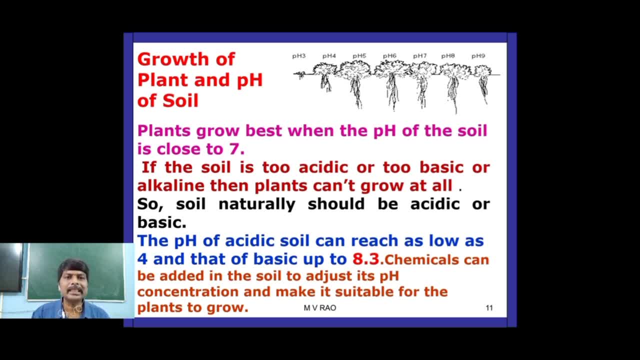 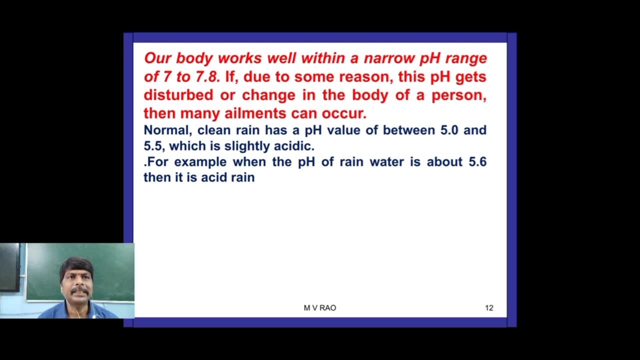 change in the body of a person then many problems can occur similarly rainwater a ph is less than 5.6 then it is called acid rain similarly aquatic life like fish can survive in lake or river water 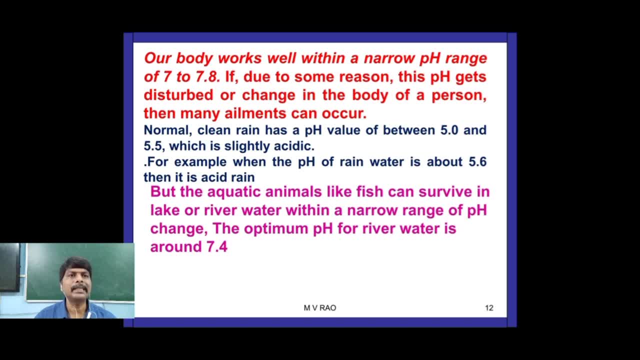 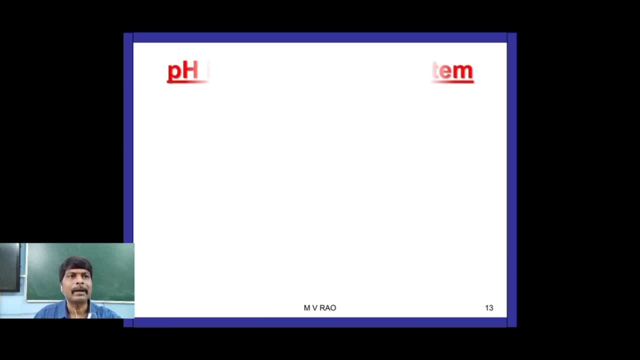 with a narrow range of ph change the optimum ph for river water is around 7.4 so for aquatic life for animals for plants ph is optimum ph is needed next coming to mankind ph in our digestive system 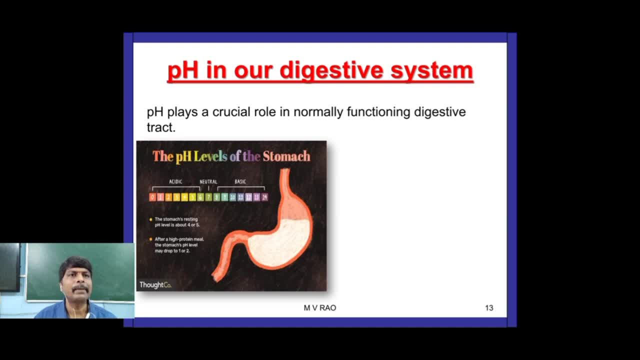 ph plays a crucial role in normally functioning digestive system in human beings now you see ph in our digestive system is a very important part of our digestive system 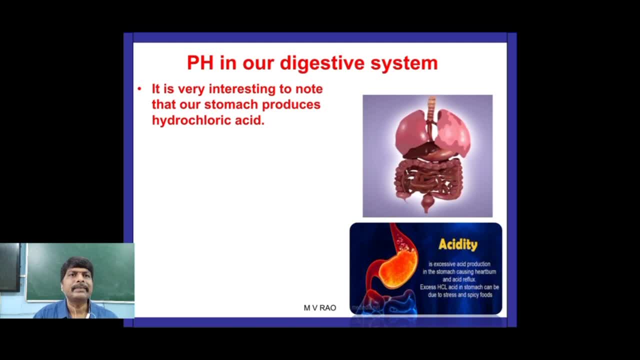 ph in our digestive system actually it is very interesting to note that our stomach produces hydrochloric acid scl hydrochloric acid is a very essential for the digestion of food it helps in digestion of food without harming the stomach it is very interesting to note that 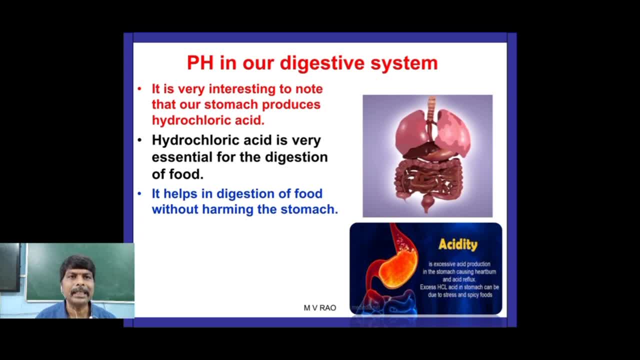 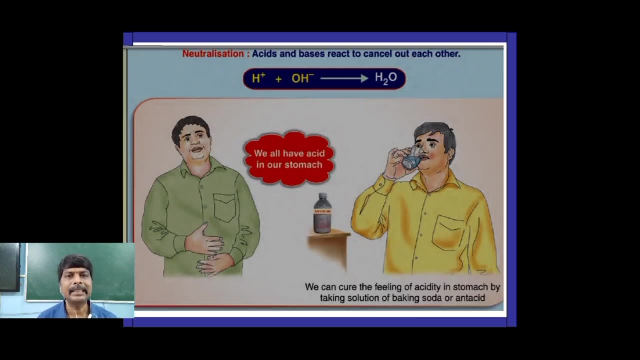 our stomach produces hydrochloric acid hydrochloric acid is very essential for the digestion of food it helps in digestion of food only without harming the stomach so if it is a more than required amount of excess of scl is there in our stomach so then the gastric problem will come acidity 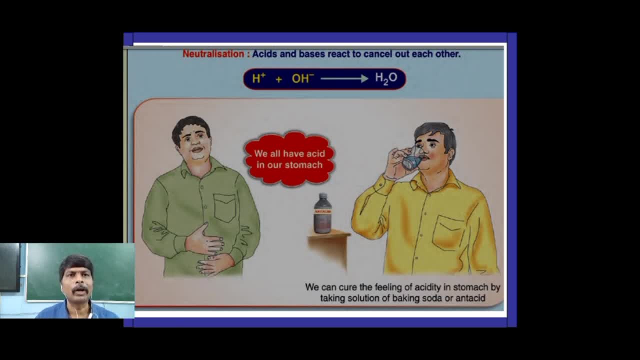 how to control that acidity that is also it will come here by neutralization 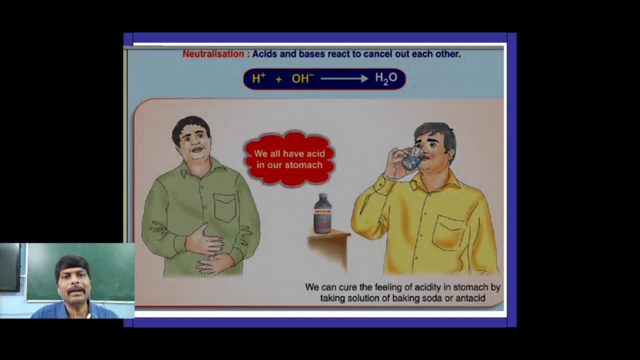 you know during neutralization acid and bases react to cancel out each other so acid and base will react together to form acid acid and base will react together in order toчик acidist standsListenna 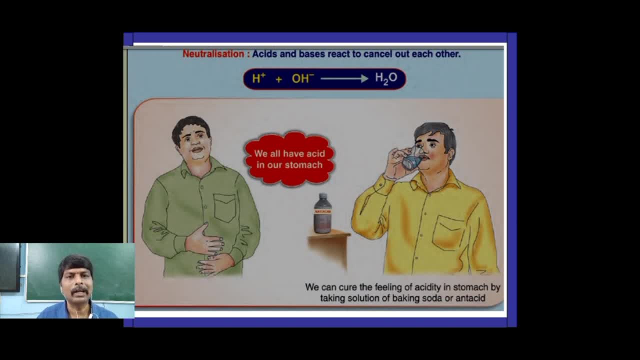 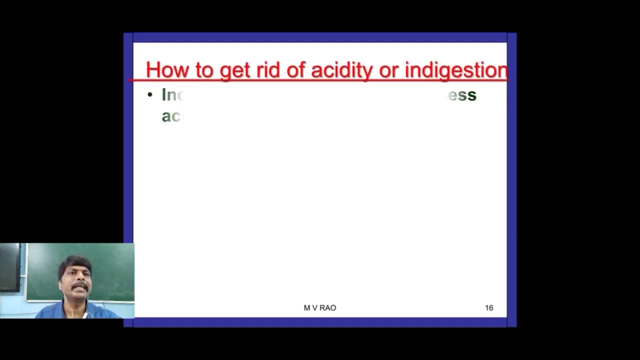 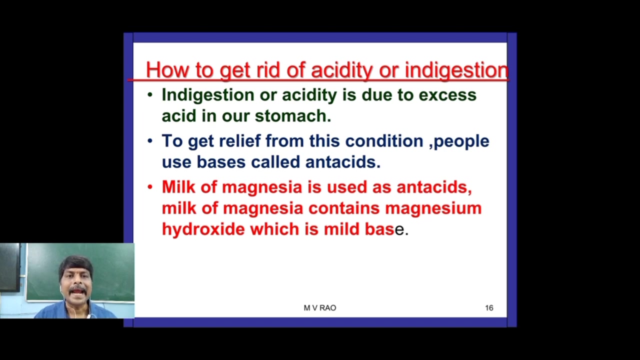 a new compound salt and water that is called neutralization chemically. In our stomach if excess production of HCL is there then they will feel gastric problem acidity. How to get rid of acidity or indigestion? Indigestion or acidity is due to excess of acid in our stomach. To get relief from this condition people use bases called antacid. Name itself it is there antacid, anti-acid. Antacids, water antacids, milk of magnesia is used as antacid. Milk of magnesia contains magnesium hydroxide which is a mild base. It reacts with excess of acid present in the stomach. 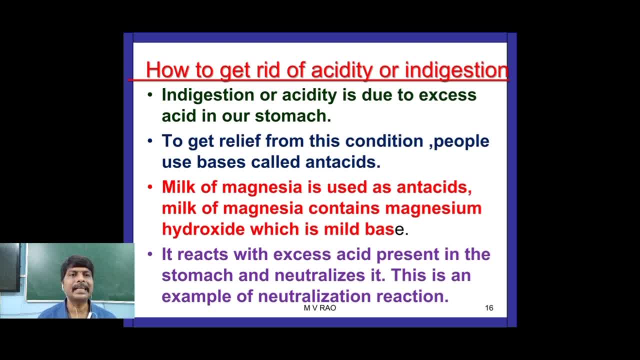 And neutralizes it. This is an example of neutralization reaction. Which substance is using as antacid? Milk of magnesia. What are antacids? These substances which are used 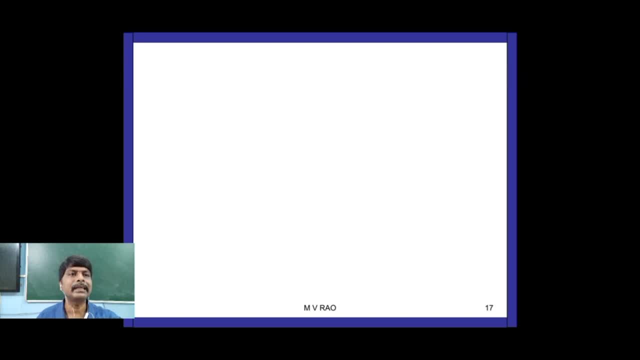 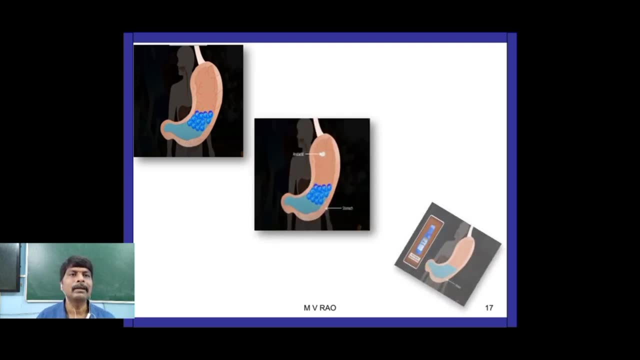 to neutralize excess of acid produced in the stomach. Now you see here acid excess is there, excess of acid produced by using antacid, that excess of acid is there. 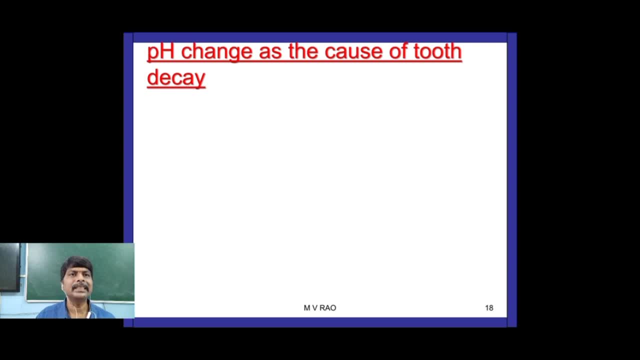 neutralized now you see ph change at the cause of tooth decay tooth decay you see the teeth here so this one will spoil because of that acids because of change in ph tooth decay starts 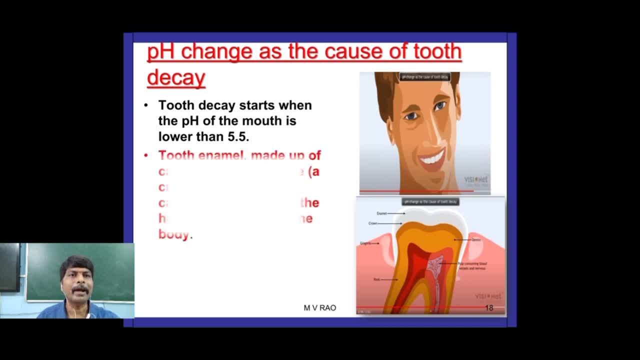 when the ph of the mouth is lower than 5.5 so lower than 5.5 means it is becoming acid 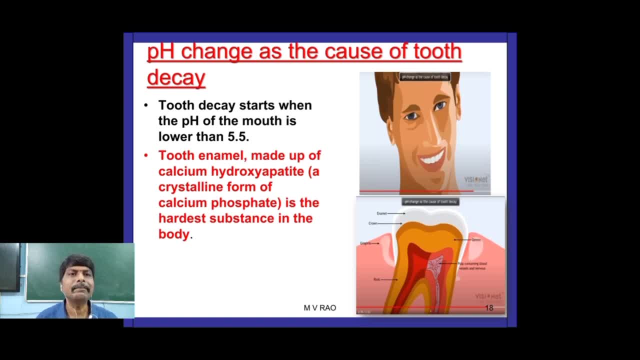 tooth enamel is made up of calcium hydroxapatite tooth enamel is made up of calcium hydroxapatite is the crystalline form of calcium phosphate is the hardest substance in the body what is the chemical name of tooth enamel calcium hydroxapatite it is a combination of calcium phosphate so it is 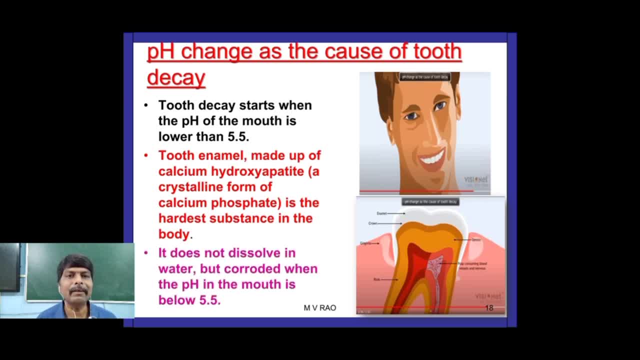 the hardest substance in the body it does not dissolve in water 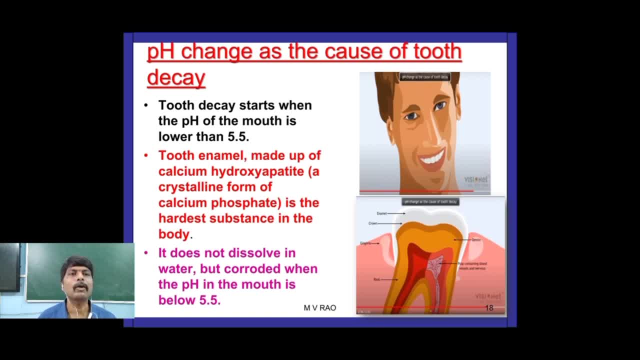 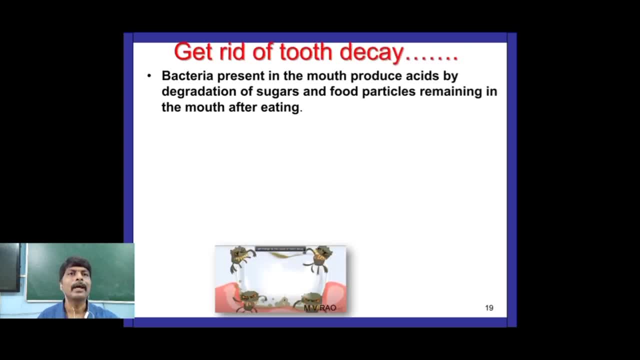 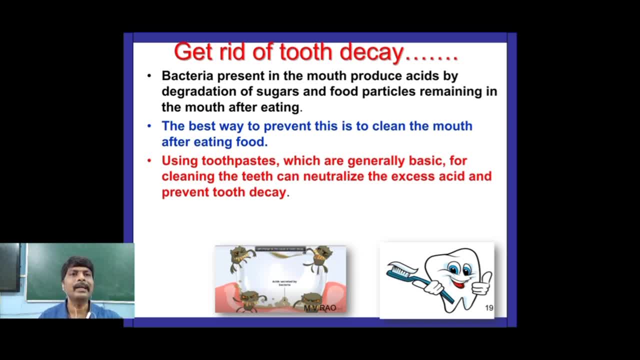 are average second goes above normal after if your heart the民 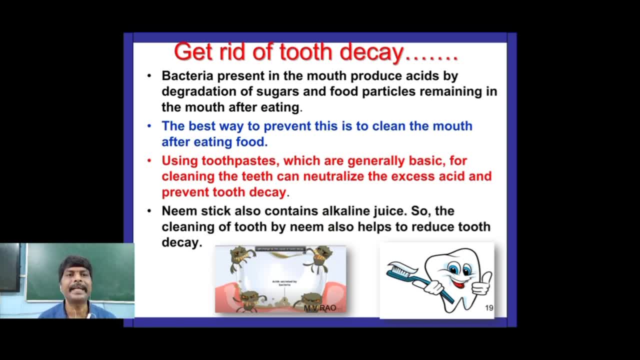 stick also contains alkaline juice that's why it is bitter neem stick also contains alkaline juice 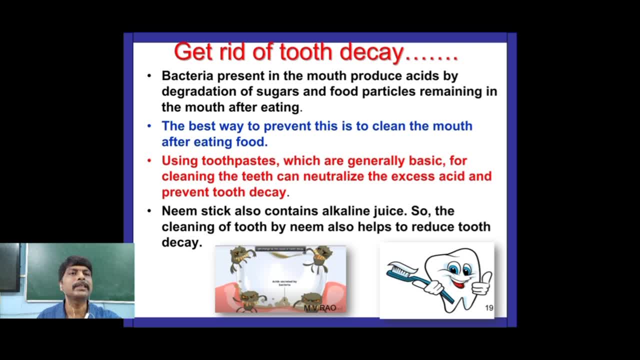 so the cleaning of tooth by neem also helps to reduce tooth decay so self depends by animals 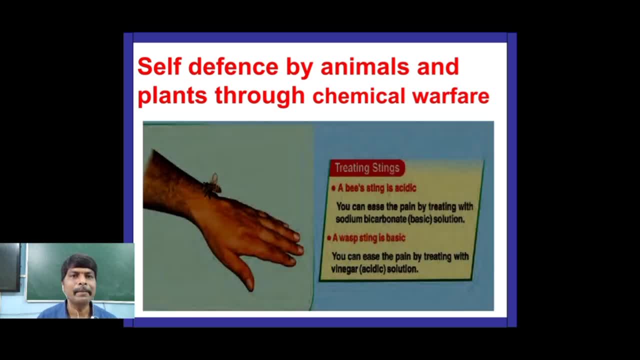 plants through chemical warfare you see any beast after bite you will feel some pain because it will 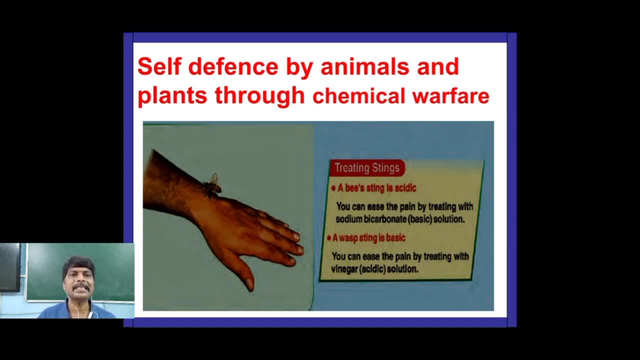 inject one acid into our body what is the acid anybody that acid is methanoic acid or formic acid methanoic acid or formic acid so it can be neutralized by applying baking soda it can be 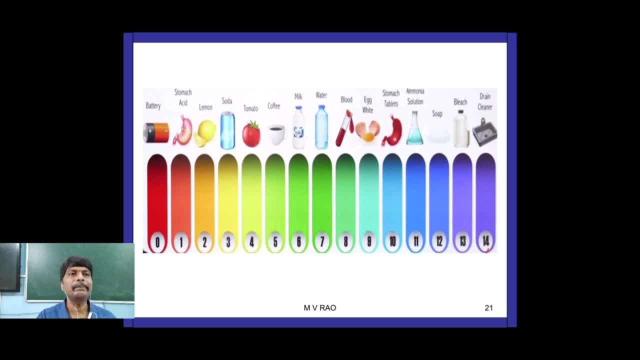 neutralized by applying baking soda so it is the ph of different substances battery acid ph is zero stomach acid ph is one lemon ph is around two so like that up to 14 different examples given 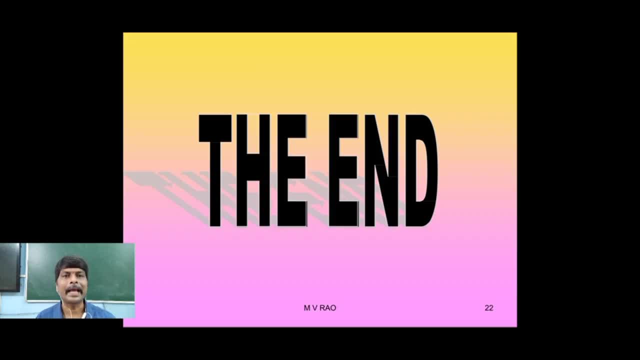 please read all these examples okay thank you you